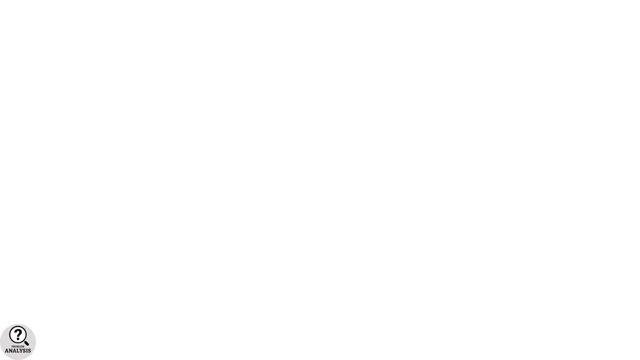 check an important point here, since- this is true problem of the square- we don't know of touching circles. Consider two circles touching each other at some point externally, Then the fact is the centers of the circles and their touching point are collinear, That is, they. 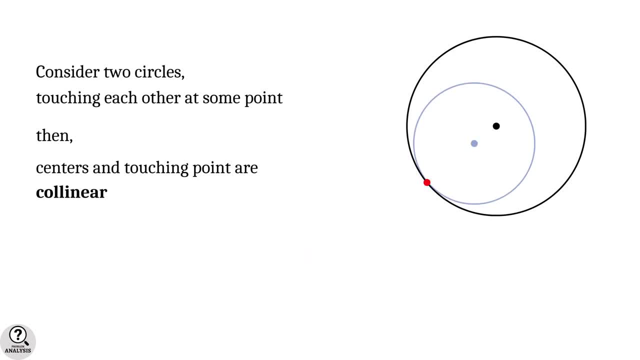 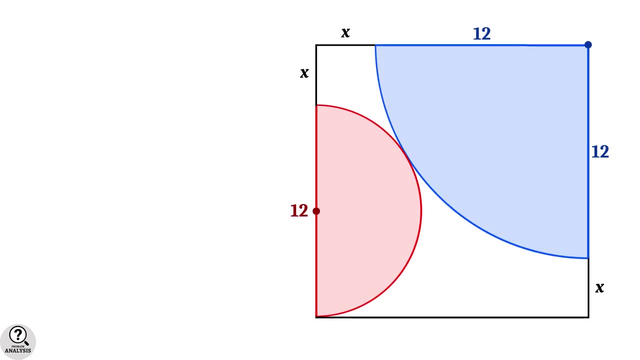 are lying on the same line. Now, if the circles are touching internally, that is, one circle inside the other- still the result is true, That is, the centers and the touching point are collinear. Now come back to our problem and mark the centers of the semicircle and the quarter circle. 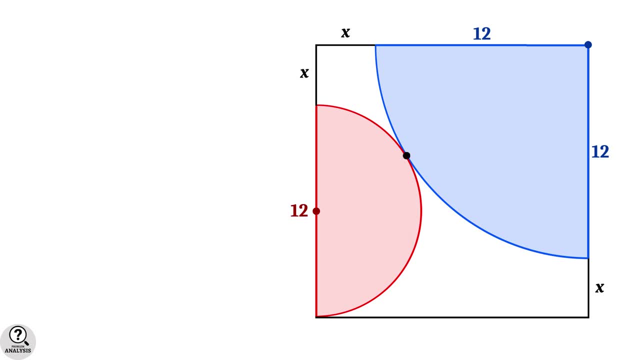 Also mark their touching point. Then, by the property we have told, these three points can be joined using a single line. Now note that diameter of the semicircle is 12 units. Then the radius will be 6 units and therefore this length, which is also a radius, is equal to 6 units. 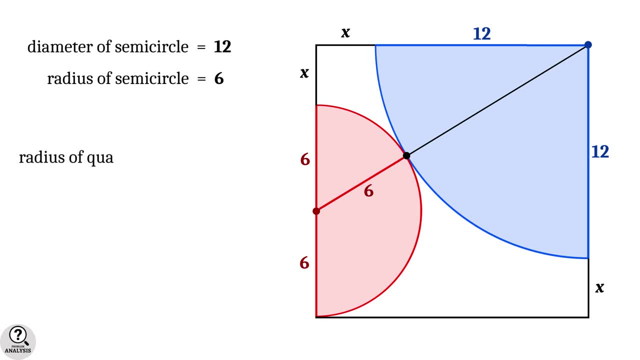 Similarly, observe the quarter circle We have. the radius is equal to 12 units. Then this length, which is also a radius, is equal to 12 units. Now we can see a right triangle here. Check the side lengths: Left edge is equal to 6 plus. 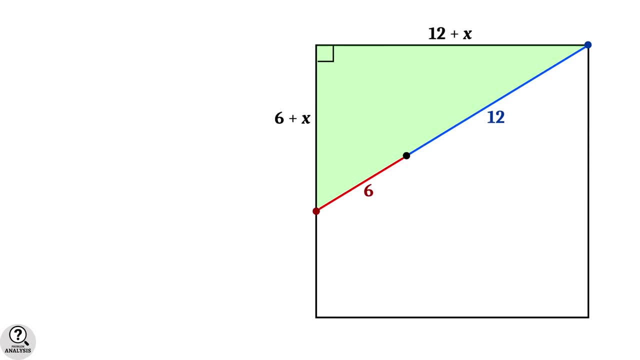 X Top edge is equal to 12 plus X and finally, the hypotenuse is equal to 6 plus 12, which is equal to 18 units. So we have a cap around both sides of this diagonal. here Now average иcance of these Eisence vectors: So what Cyx is equal to? This length is equal to 12i plus ix and finally, the hypotenuse is equal 6 plus 12i, also equal 12u. The covariance is equal to 18 units. There are 13真ie and 14 осnes that are between the 5 and 10U terms. 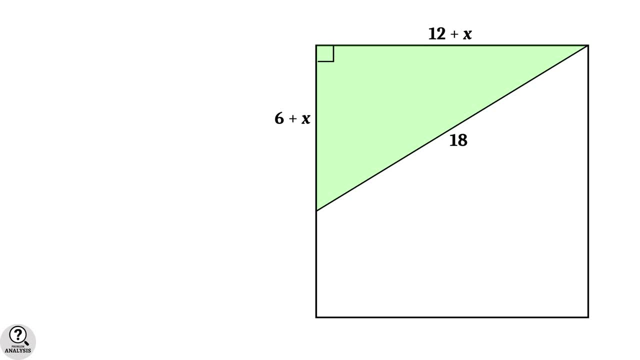 Now everything is just a matter of calculation. Here we have a right triangle with all the edges are given. So apply Pythagoras theorem. It will give. 6 plus x whole square plus 12 plus x whole square is equal to 18 square. 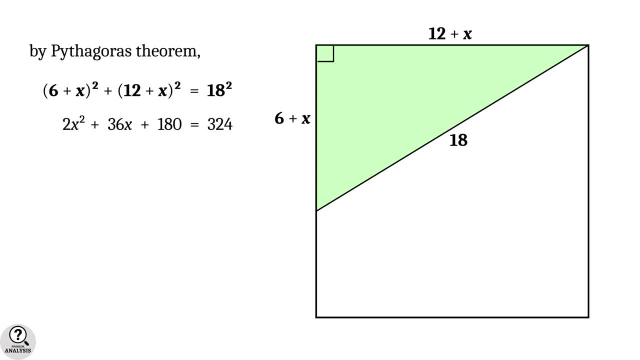 Further simplification will give 2x square plus 36x plus 180, equal to 324.. That is x square plus 18x minus 72, equal to 0.. Now solve this quadratic equation to obtain the value of x. For a general quadratic equation of the form ax square plus bx plus c, equal to 0,, we have: